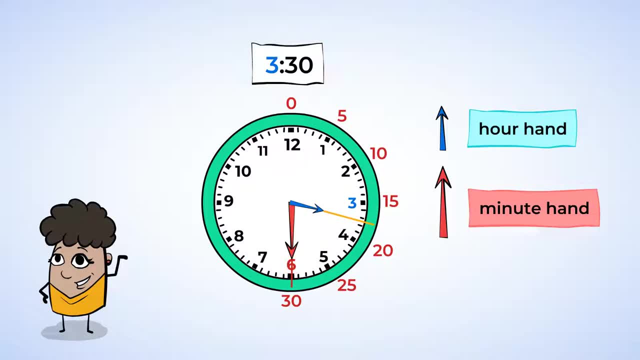 So the long hand points to the 6. When the clock looks like this, we know it's 3.30.. And it's movie time. And now we know how to read an analog and a digital clock Right, Except that it isn't yet 3.30.. 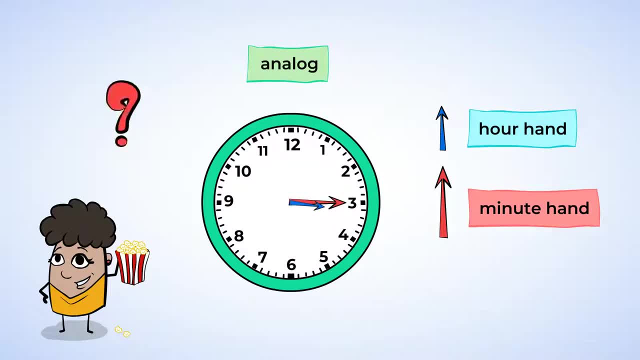 This is the actual time, So let's figure out what time it is. First, look at the hour hand. OK, the hour hand is still pointing between the 3 and the 4. And that means the hour is 3.. And now let's look at the minute hand. 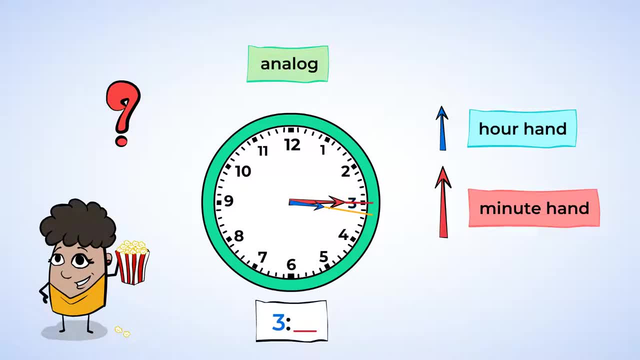 OK, the minute hand is right on the 3. We have to figure out how many minutes that means. Well, we know that there are 60 minutes in an hour, And so we can skip count by fives to figure this out. 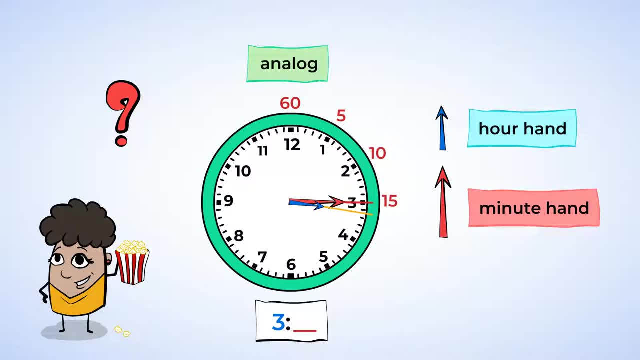 5,, 10, 15.. So there are 15 minutes And this means it must be 3.15.. Awesome, Not too long until it's movie time. That was really cool how we could skip count by fives to help figure out the time. 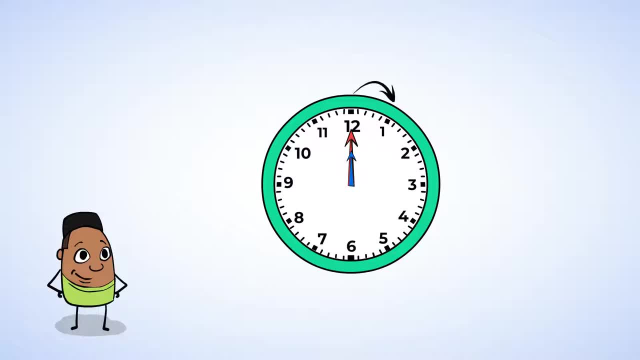 And this is because the space between every two numbers on a clock represents 5 minutes. The clock shows 12 o'clock right now, So starting there, You can skip count by fives around the clock, like this: 12.05,, 12.10,, 12.15,, 12.20,, 12.25,, 12.30,, 12.35,, 12.40,, 12.45,, 12.50,, 12.55. 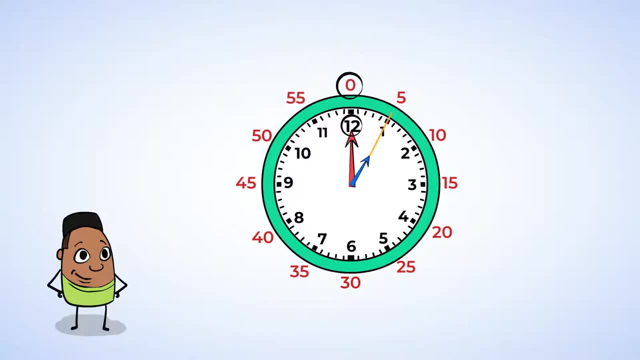 Then, instead of 60,, a new hour begins and we're back to zero minutes, And in this case it's one o'clock. Now let's use what we've just learned and practice. This is telling time on a few different clocks. 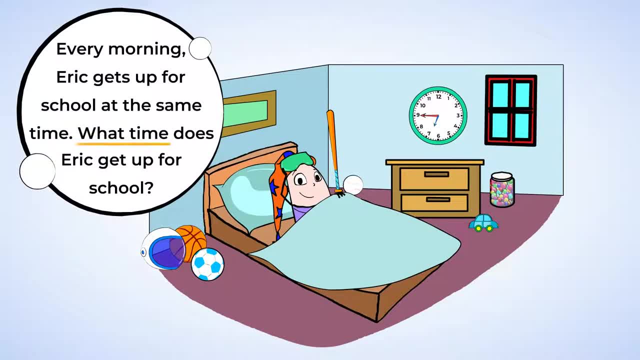 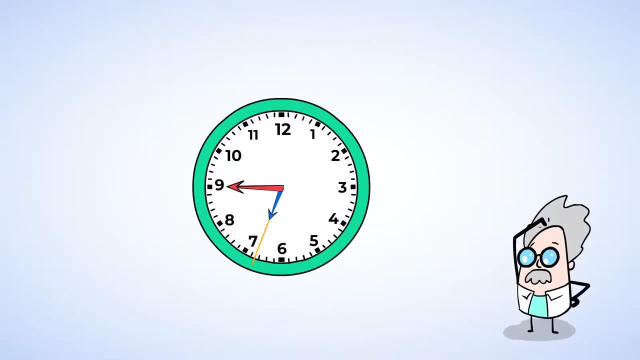 Every morning, Eric gets up for school at the same time. At what time does Eric get up for school? First, let's look at the hour hand. We can see that it's between the 6 and the 7.. So the hour is that's right, 6.. 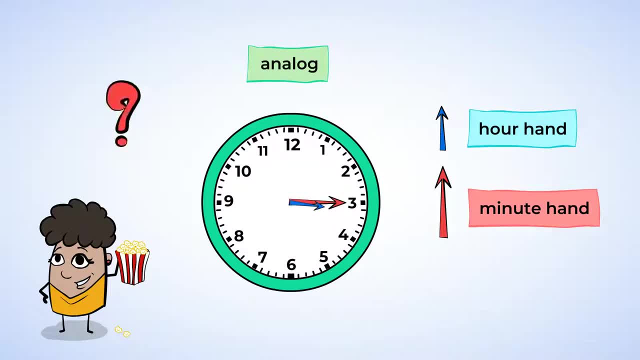 This is the actual time, So let's figure out what time it is. First, look at the hour hand. OK, the hour hand is still pointing between the 3 and the 4. And that means the hour is 3.. And now let's look at the minute hand. 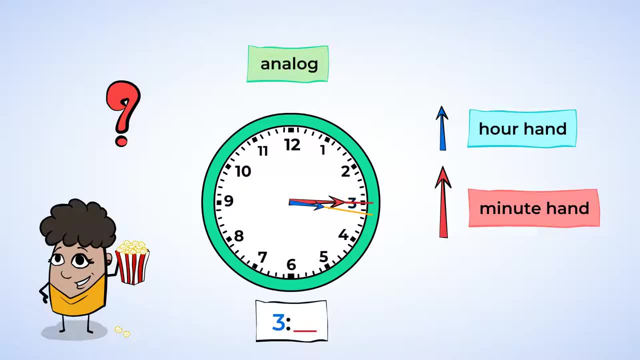 OK, the minute hand is right on the 3. We have to figure out how many minutes that means. Well, we know that there are 60 minutes in an hour, And so we can skip count by fives to figure this out. 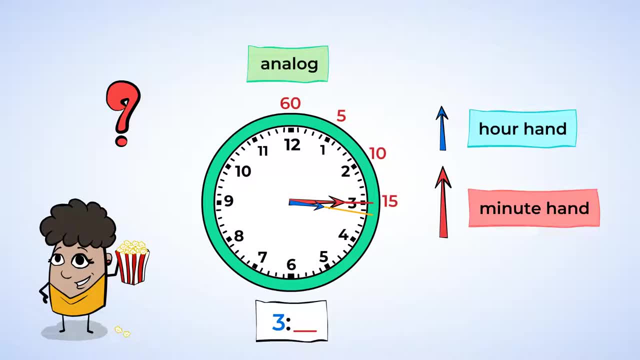 5,, 10, 15.. So there are 15 minutes And this means it must be 3.15.. Awesome, Not too long until it's movie time. That was really cool how we could skip count by fives to help figure out the time. 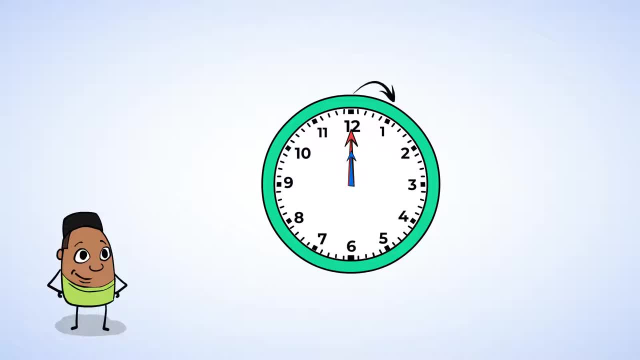 And this is because the space between every two numbers on a clock represents five minutes. The clock shows 12 o'clock right now, So we can figure out how many minutes it is. So, starting there, you can skip count by fives around the clock, like this: 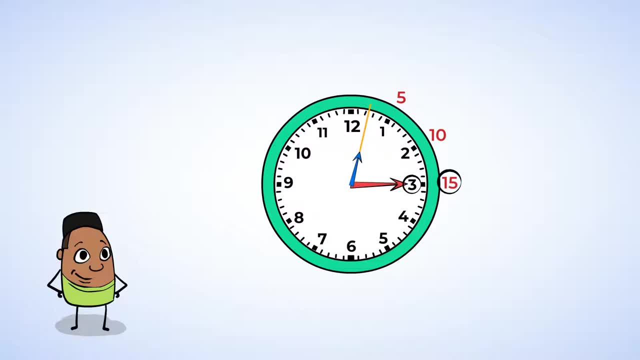 12.05, 12.10,, 12.15,, 12.20,, 12.25,, 12.30,, 12.35,, 12.40,, 12.45, 12.50, 12.55.. 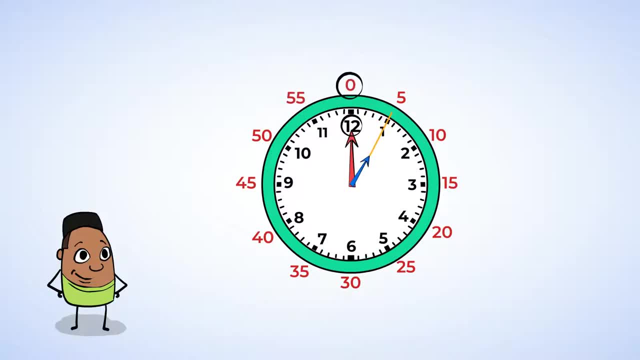 Then, instead of 60,, a new hour begins and we're back to zero minutes, And in this case it's 1 o'clock. Now let's use what we've just learned And practice telling time on a few different clocks. Every morning, Eric gets up for school at the same time. 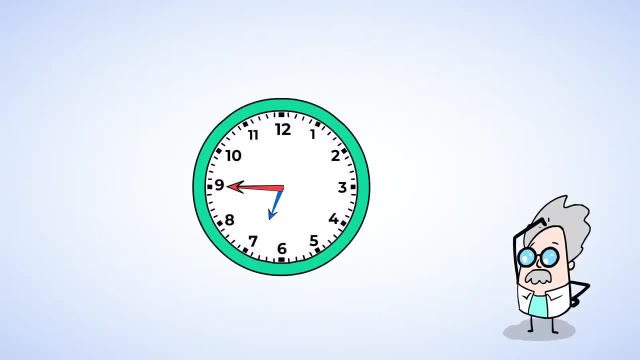 At what time does Eric get up for school? First let's look at the hour hand. We can see that it's between the 6 and the 7. So the hour is that's right, 6.. Next look at the minute hand. 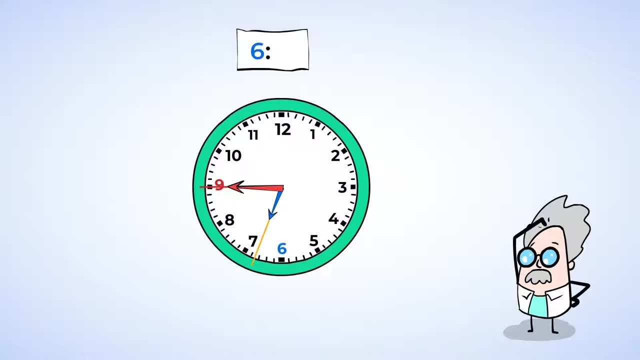 It's on the 9.. Now you might remember how many minutes 9 represents, But if you don't, you can always count by fives, So let's do that. Starting from number one on the clock, we have 5,, 10,, 15,, 20,, 25,, 30,, 35,, 40,, 45.. 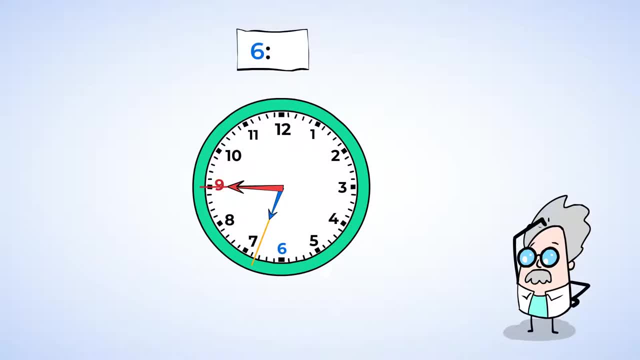 Next, look at the minute hand. It's on the 9.. Now you might remember how many minutes 9 represents, But if you don't, you can always count by 5.. So let's do that. Starting from number 1 on the clock, we have 5,, 10,, 15,, 20,, 25,, 30,, 35,, 40,, 45.. 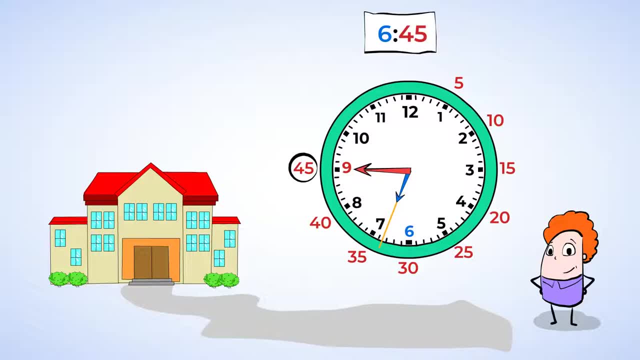 So Eric gets up at 6.45 for school, Oh, but does Eric get up at 6.45 am or 6.45 pm? Oh, am and pm help us to identify the section of the day. 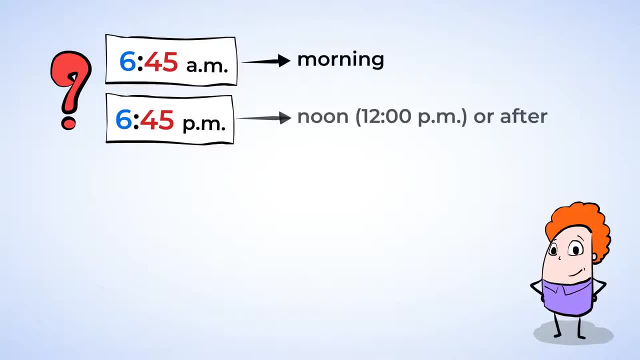 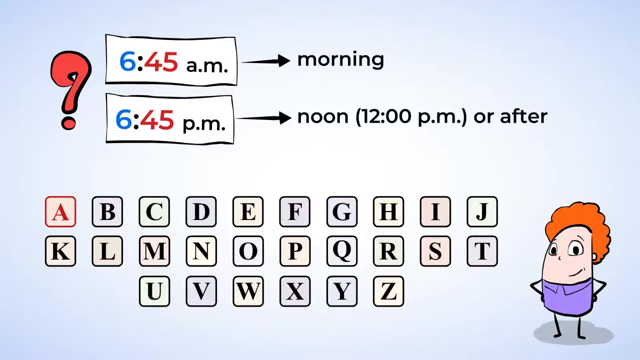 Am is for the morning and pm is noon or 12 pm and everything after Now. here's a way to help you remember: A comes before p and therefore am comes before pm. So does Eric get up for school at 6.45 am or 6.45 pm? 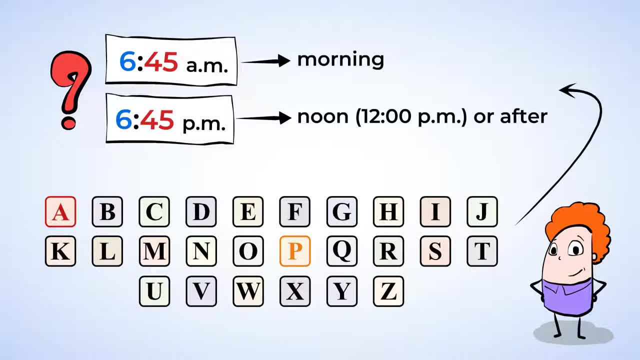 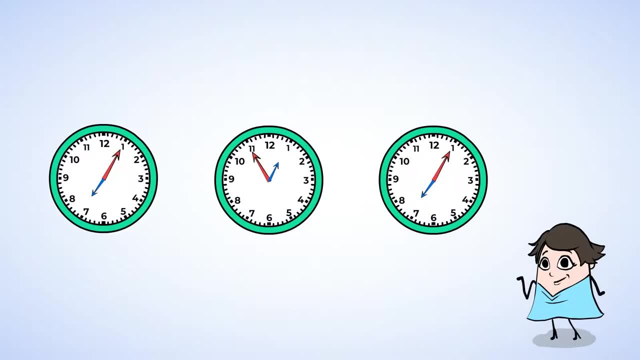 Well, he gets up for school in the morning, so we know that Eric gets up for school at 6.45 am. Great work. Now the clocks below show when Eric eats: breakfast, lunch and dinner, And here are three different times. 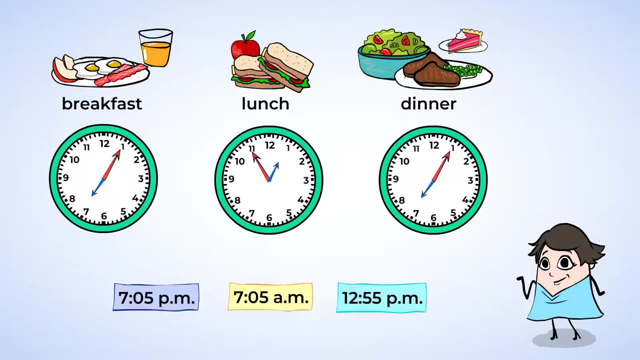 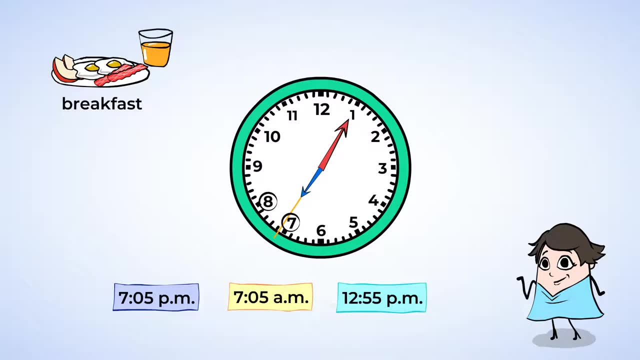 Uh-huh, Let's match the times to the correct clocks. First breakfast: We can see the hour hand is between the 7 and the 8. And this means the hour is 7. And the minute hand is on the 1, so this means 5 minutes. 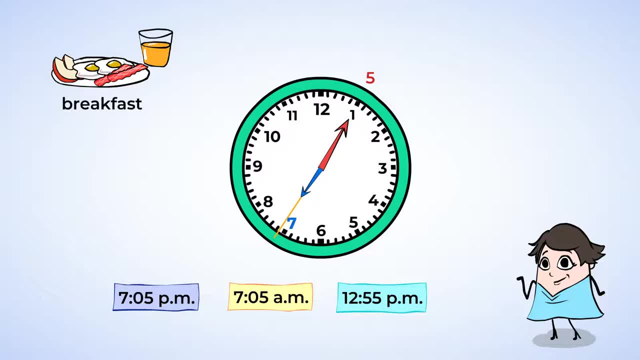 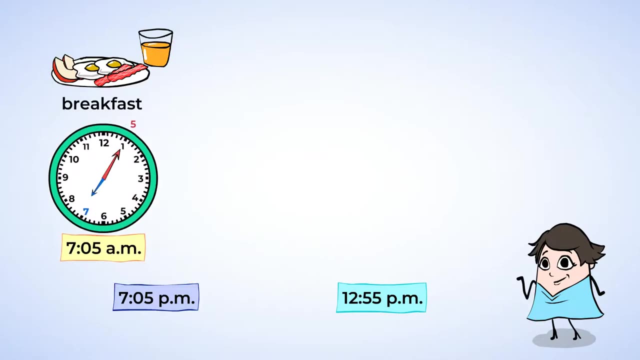 So breakfast time is Ooh, but there are two 7.05 answer choices: 7.05 am and 7.05 pm. Wait, breakfast is in the morning, so 7.05 am. Great job. 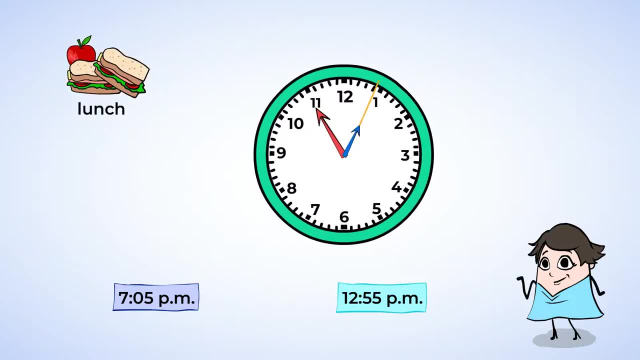 Next is lunchtime. This hour hand is close to the 1,, but not quite. Uh-huh, That means that the hour is still 12.. The minute hand is on the 11. 11.. If you forget how many minutes that is, don't worry. 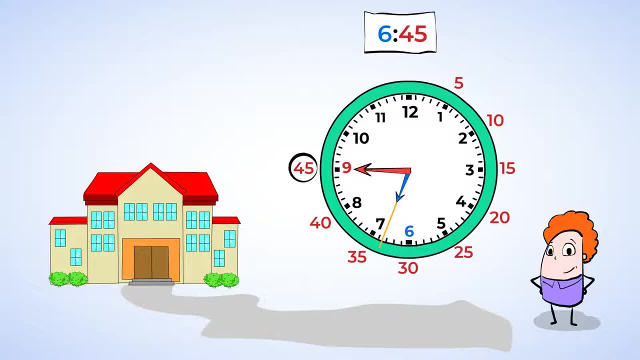 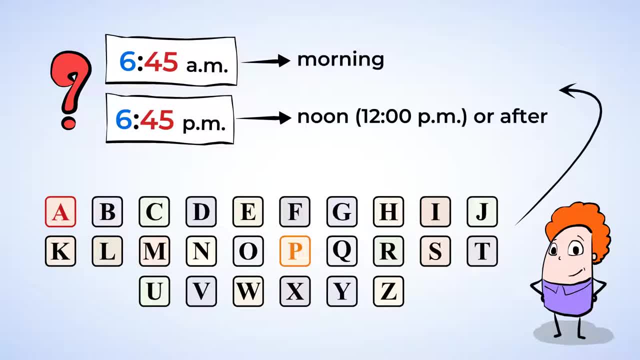 Am is for the morning and pm is noon or 12 pm and everything after Am comes before pm. So does Eric get up for school at 645 am or 645 pm? 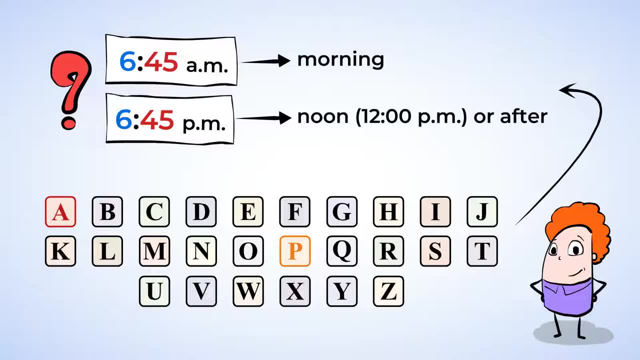 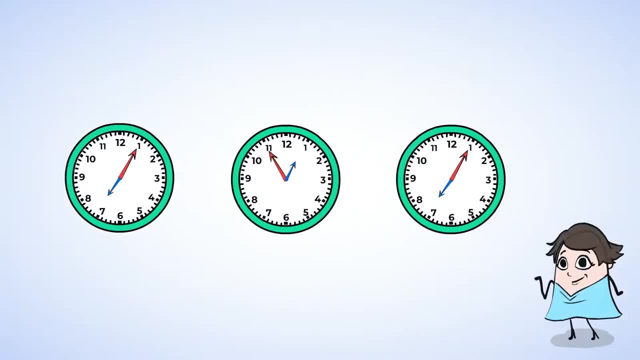 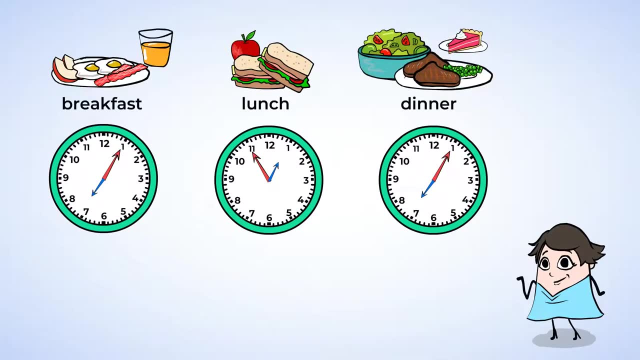 Well, he gets up for school in the morning, so we know that Eric gets up for school at 645 am. Great work. Now the clocks below show when Eric eats: breakfast, lunch and dinner, And here are three different times. 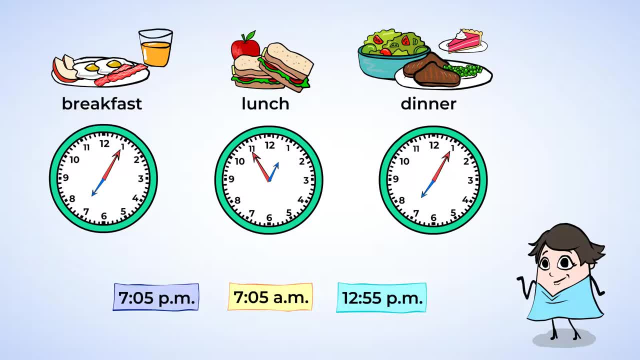 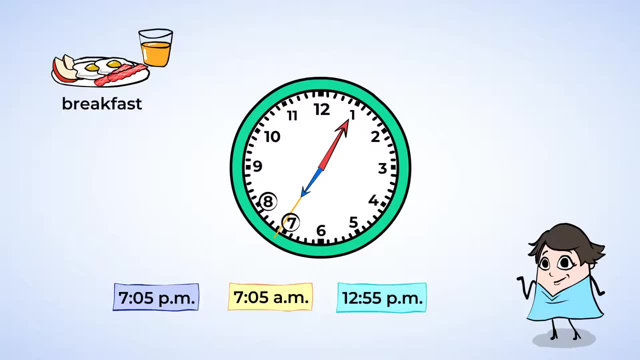 Uh-huh times to the correct clocks. First breakfast. We can see the hour hand is between the 7 and the 8, and this means the hour is 7.. And the minute hand is on the 1, so this means 5 minutes. So breakfast time is 7.05.. Oh, but there are. 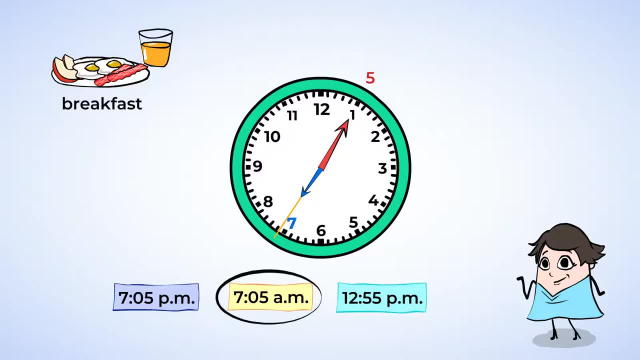 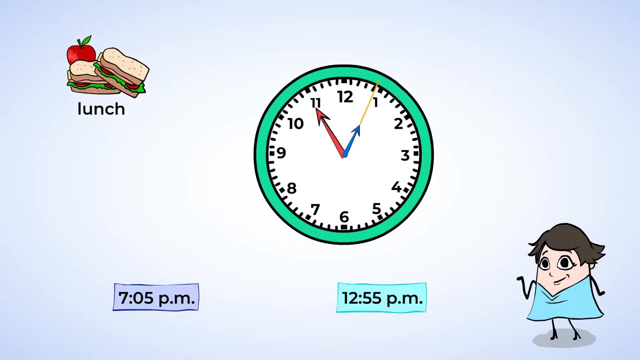 two 7.05 answer choices: 7.05 am and 7.05 pm. Wait, breakfast is in the morning, so 7.05 am. Great job. Next is lunchtime. This hour hand is close to the.